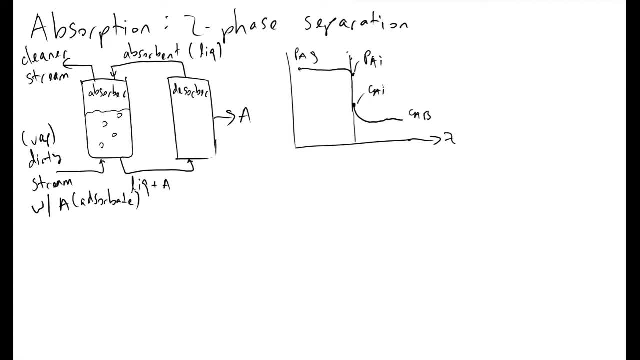 neglecting curvature in this example, And we can now ask ourselves: what kind of mass transfer or flux can we be observing in this system? And so what we'll do is we'll define two regions and we'll note that the flux of A in our 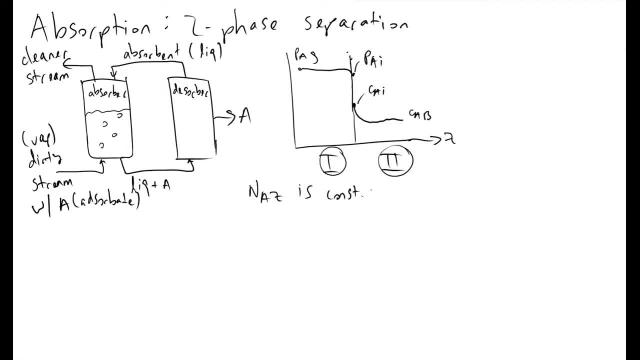 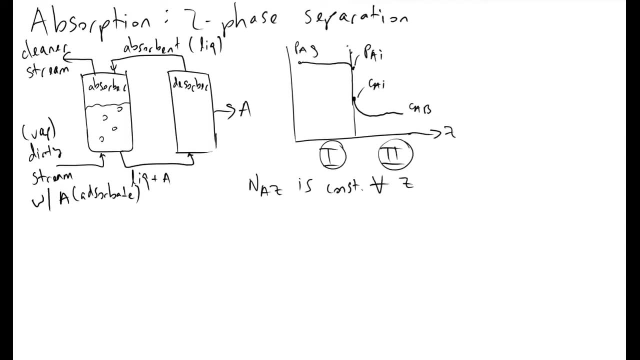 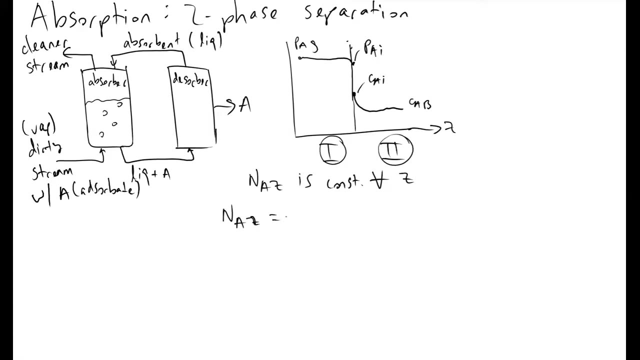 Z direction is constant for all Z because mass is conserved and we have no accumulation. And by doing that what we can define our flux to be in AZ is some local mass transfer coefficient called little k, g in our gas phase times the bulk concentration of the bulk partial pressure of A in the gas phase minus the interfacial partial pressure of A, and this term must also be equal to a local mass transfer coefficient in our liquid phase, called little k sub l, and that has a driving force of distel. KG in our phase minus the interfacial partial pressure of A, And this term must also be equal to a local mass transfer almighty. thank you to the self'll be workingwohl her�, Her instructors, an a or we also have some in Carletonortion had big company of him who will help you on your work And we will see child, as you have seen, tomorrow time He personally gets familiar insh. 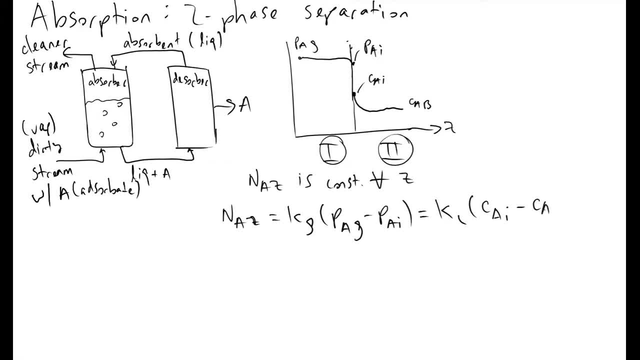 C-A-I minus C-A bulk. The problem at this point is we do not know what P-A-I or C-A-I are. They're very difficult to measure because we can't very easily extract the solution at the interface between these two species. So what we are going to do is we're going to define. 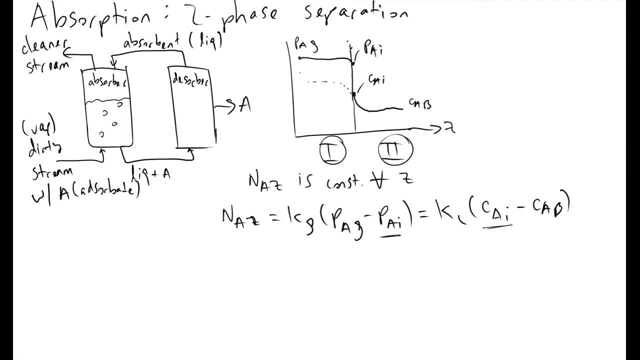 some fictitious quantities and call them C-A star and P-A star. And the reason we define these quantities C-A star and P-A star is because they will allow us to invoke a global mass transfer coefficient and pretend as if so, if we had a liquid global 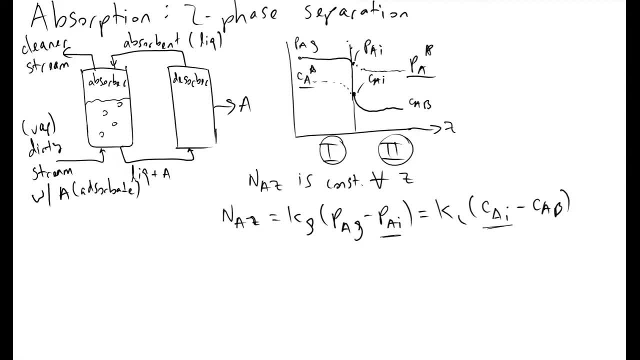 mass transfer coefficient, we could evaluate or claim that the driving force would be equivalent to C-A star minus C-A bulk. And in the case of a global gas mass transfer coefficient, we could say its driving force would be P-A-G minus P-A star. 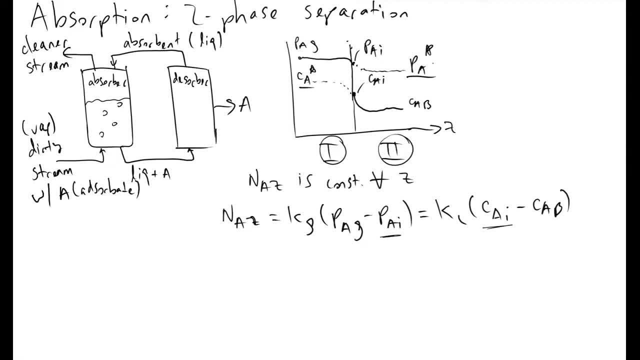 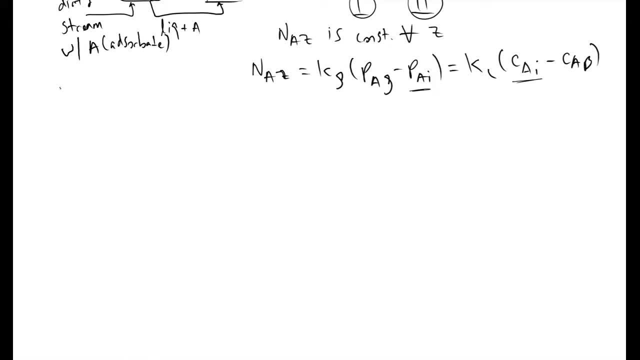 And to actually evaluate what P-A star and C-A star are, we turn to equilibrium data that we will have because it's tabulated or we can evaluate it experimentally, And if we look at equilibrium curves for our species A, because we'll know what we're working with or what we 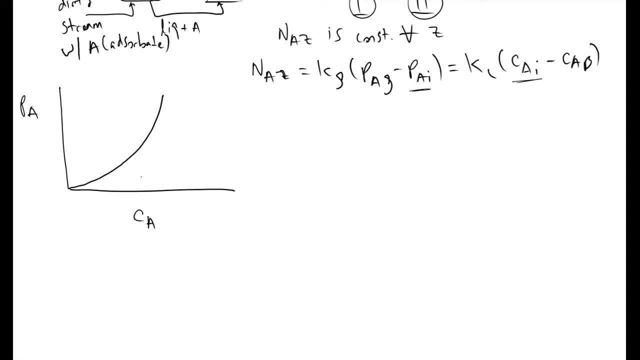 want to extract versus its concentration. So if we plotted the composition of A in the gas phase as well as in the liquid phase at various compositions, we would get some kind of equilibrium data that looks like this: What we would see is that if we knew what our composition of C-A in the bulk is, if we draw a line up from that, 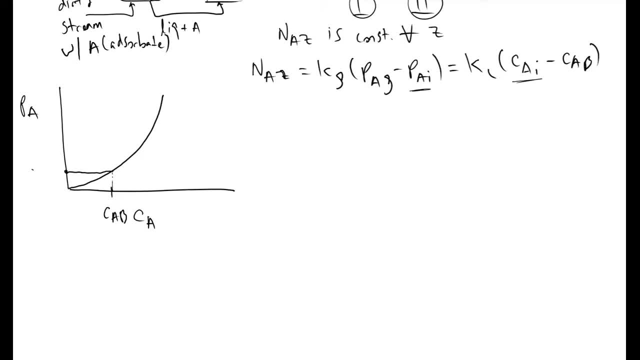 and then look to the left, we will find what the fictitious quantity P-A star would be. And then, if we knew well, we would know what the composition or the partial pressure of A is in our gas phase. we can define what the 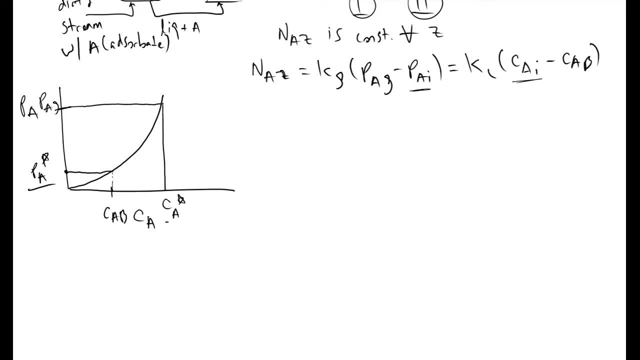 fictitious quantity C-A star would be. And having done that, we can now use our global mass transfer coefficients big K-G and big K-L. And before I do that, I'd like to say how we might get this equilibrium curve. 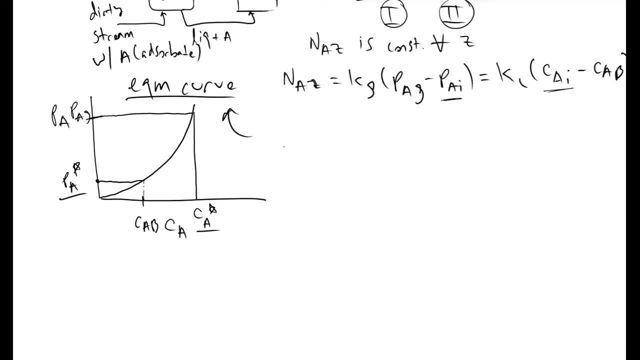 This equilibrium data can come from. if you took Excel and you had some kind of data that told you the partial pressure of A in a liquid- sorry, the partial pressure of A in a gas and the partial pressure or the concentration of A in a liquid, you would have values, And this is just an xy chart. 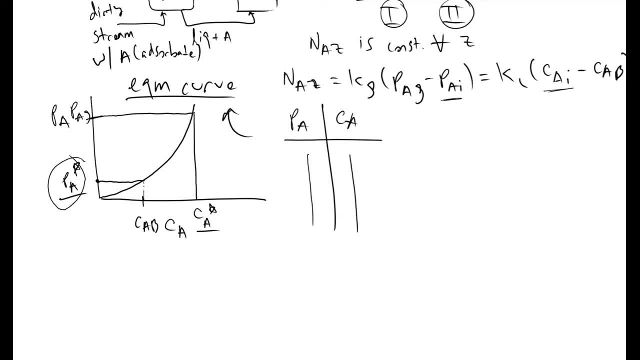 and you could pretty easily graph this to find P-A star in C-A. And so now, getting back to the global mass transfer coefficients, we will define our flux in the z-direction to be big K-G times, P-A-G minus P-A star. 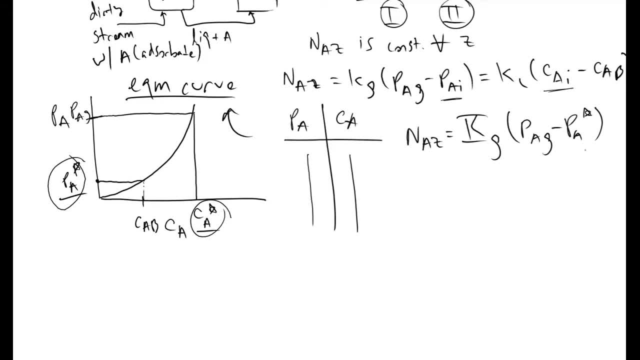 as if we assume that instead of a liquid on the outside of our bubble, we have a big K-G. As if we assume that instead of a liquid on the outside of our bubble we have a big K-G bubble. we had a vapor, and this must also be equal to the global. 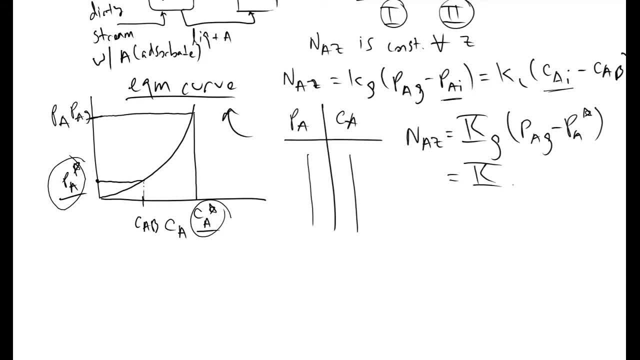 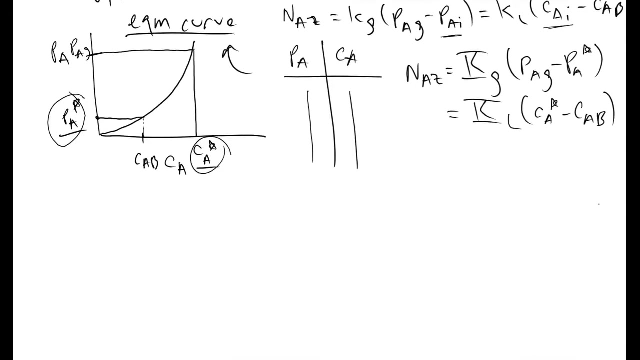 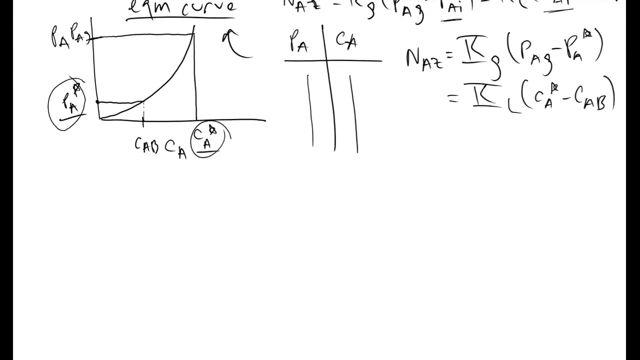 mass transfer coefficient in your liquid phase times, CA star minus CA bulk in your liquid. And what we will do now is divide big KG by big KL and use some definitions that we would have in textbooks to figure out what our equilibrium curve will look like if we could neglect curvature And so doing. 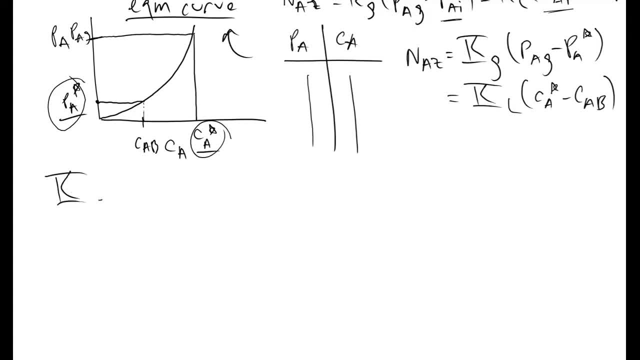 that what we would have is big KG divided by big KL and the small KG divided by the small K. Now, using the definitions that we have just gotten here, we will write this as: CA star minus CA bulk divided by PA, the partial pressure of A and the bulk of the gas minus PA star, And from textbooks this: 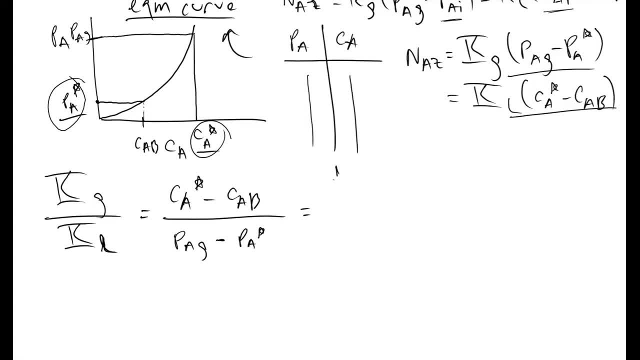 this is our equilibrium curve And then this is our equilibrium graph. so for the. this is our equilibrium graph. so for the equilibrium graph, so for the. This will have a relation of 1 over m little m kg, the local gas phase coefficient and 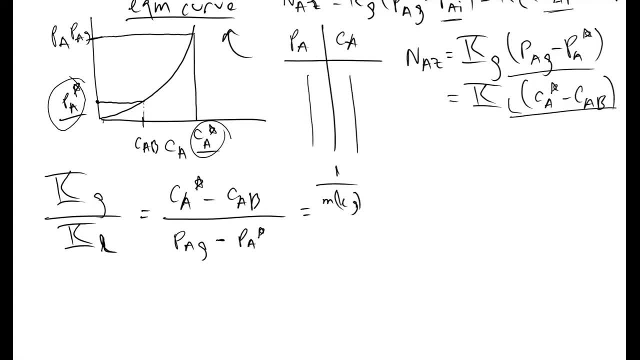 then this little m is the slope. if we were to approximate our equilibrium curve as linear, This has a slope, little m, and the numerator is 1 over. and then the local liquid mass transfer coefficient, little kl, then divided by 1 over local gas phase mass transfer coefficient. 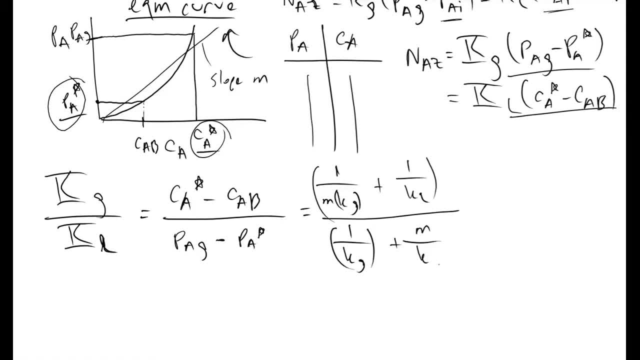 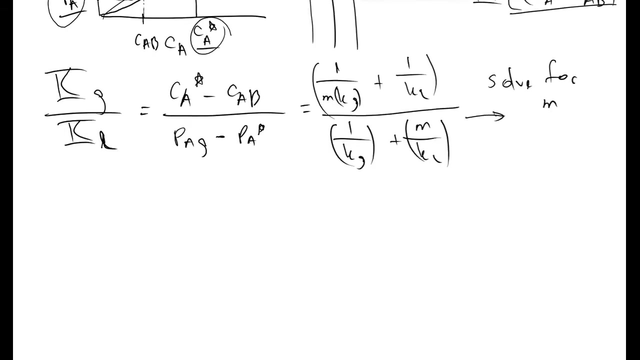 plus m over local liquid phase mass transfer coefficient And with this equation, typically you will be given values of kl and kg. so we can now solve this for m And once we know what our value of m is, we can now evaluate what our value of m is. 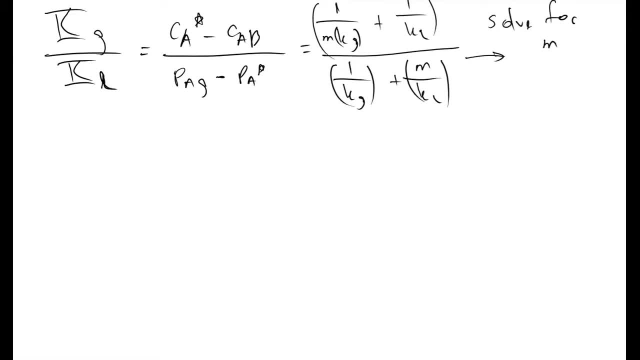 So if we want to know what our value of big Kg, the global mass transfer coefficient, in our gas phase is- this is another textbook relationship you can look up. It tells us that 1 over big Kg is equal to 1 over the local gas phase mass transfer coefficient. 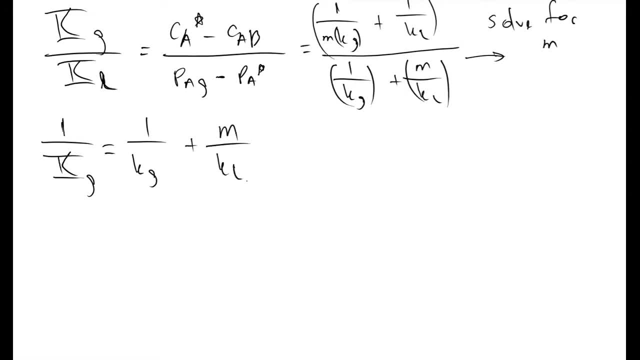 plus m over the local liquid phase mass transfer coefficient, as well as 1 over the global liquid phase mass transfer coefficient. This is the global mass transfer coefficient. It must be equal to m over the global liquid phase mass transfer coefficient, So 1 over m times the local gas transfer mass transfer coefficient plus 1 over kl. 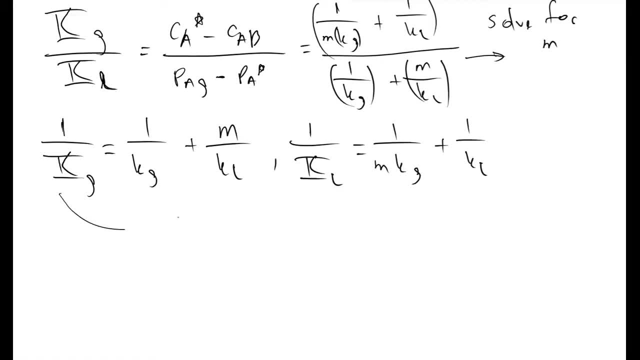 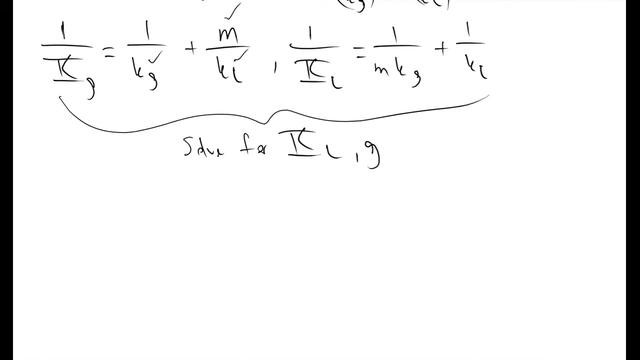 And once we evaluate these two equations, we solve for the global mass transfer coefficients. Once we have done that, because we will know what m is, kl is, kg is, We can now find what the interfacial composition is in our system. by saying that, because we 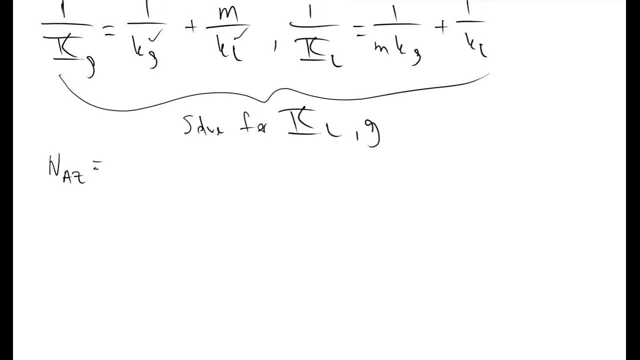 know that the flux in our z direction has to be a constant value, which would be equivalent to big Kg times the total or the bulk partial pressure of big Kg times the total mass transfer coefficient of A in your gas phase, minus the fictitious quantity PA star that we evaluated this term. 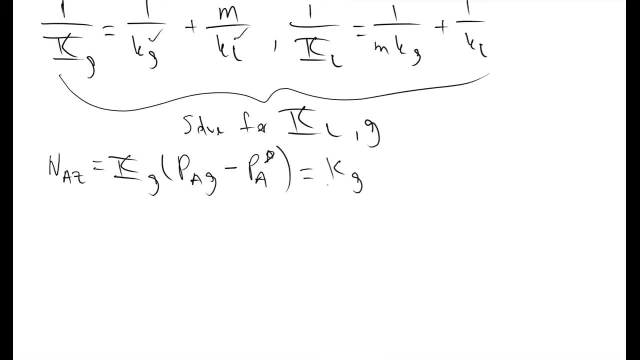 must also be equal to the local mass transfer gas coefficient times the bulk partial pressure minus the interface partial pressure, PAI. And so, once we know- because we will know every term on the left side of this equation and we know two of the three terms on the right-hand side of